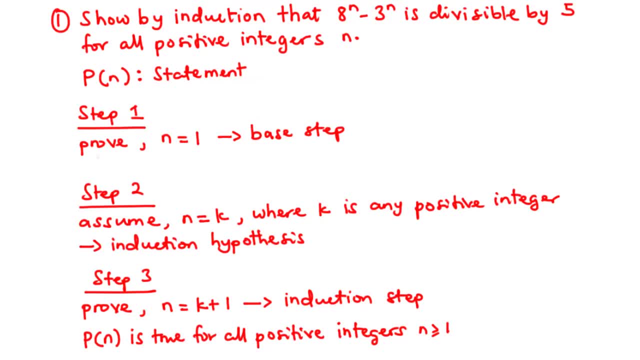 So let's try this induction problem. Show by induction that 8 exponent n minus 3 exponent n is divisible by 5 for all positive integers n. Now to solve this problem, we first of all need to know what induction is all about. Mathematical induction is basically one of the techniques. 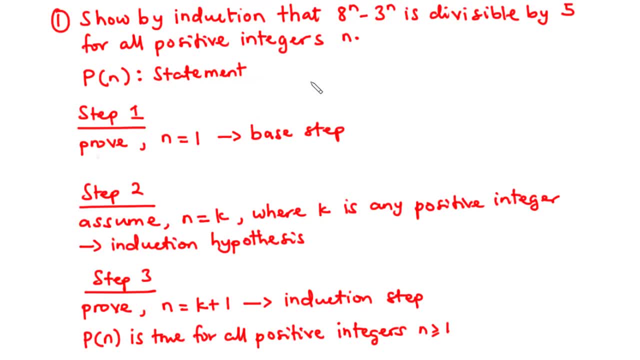 which can be used to prove a variety of mathematical statements which are formulated in terms of n, where n is a positive integer, So giving a statement, say p of n, involving the natural number n. there are basically three steps that we need to go through Now. the first step is: 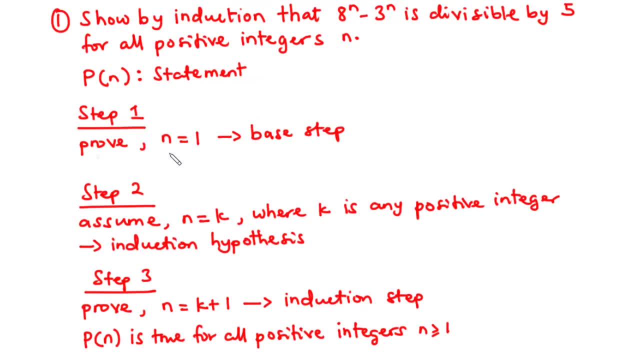 where we need to prove that the statement is true for the first time, that is, when n is equal to 1, and we call this the base step For step 2, we are going to assume that the statement is true for n equals k where k is any. 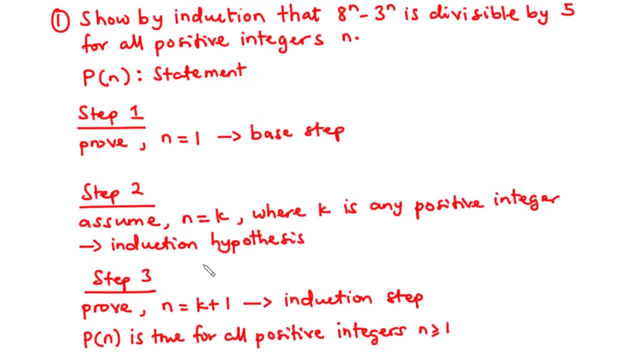 positive integer, and we call this the induction hypothesis. Now, in step 3,, based on the hypothesis made in step 2, we are going to prove that the statement is true for n equals k plus 1, that is the next step and we call this the induction step. Then we can make a statement. 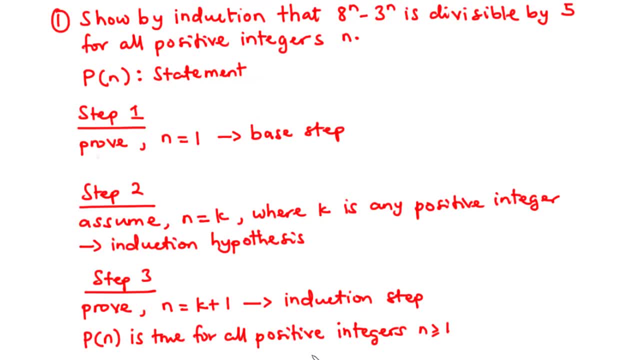 that p of n is true for all positive integers: n is greater or equal to 1.. So, basically, these are the steps that we need to follow when we want to solve problems concerning mathematical induction. So, having this in mind, let's try this problem. 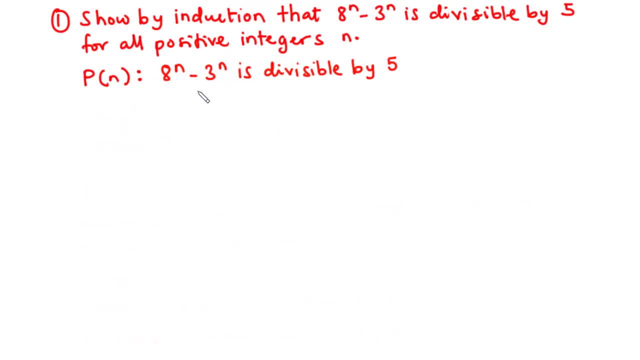 So, given the statement, 8 exponent n minus 3 exponent n is divisible by 5, now what this primarily means is that when 8 exponent n minus 3 exponent n is divisible by 5, then this is equal to some integer value, say l. Now we can simplify this as 8 exponent n minus. 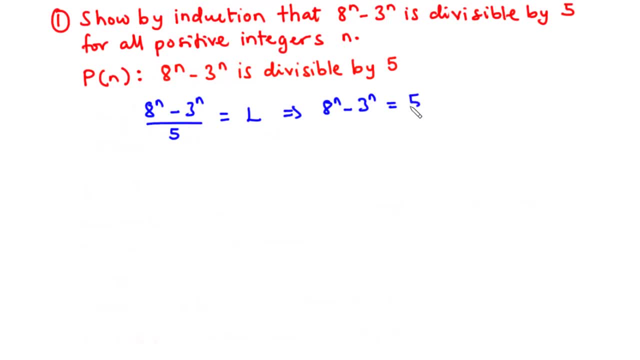 3 exponent n equals 5 times some integer value, l. For example, if we have the value 50. When 50 is divided by 5, we have some integer value 50, which is a positive integer value. So when 8 exponent n minus 3 exponent n is divisible by 5, then this is equal to some integer. 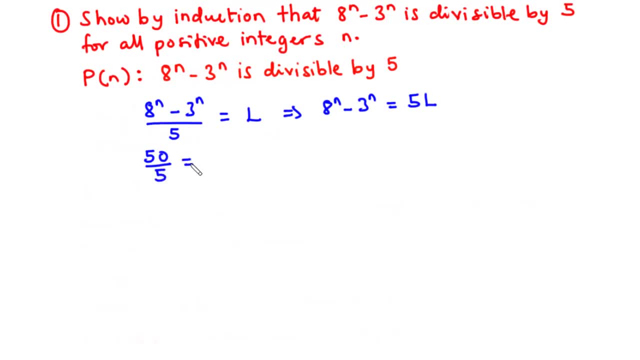 divided by 5, then the result is equal to some integer value, say l, which is equal to thing. now we can simplify this as 50 equals 5 times some integer value, say l. so this is exactly what we are talking about here. now, if we are able to prove this, 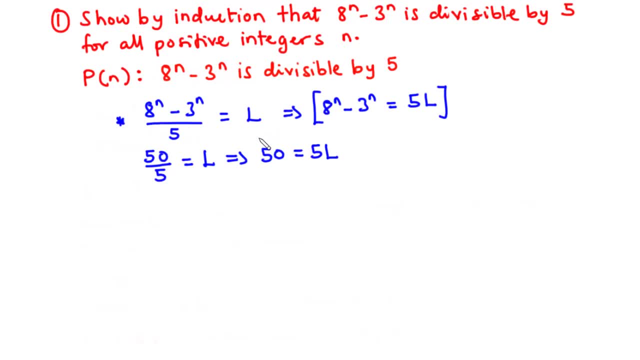 then it means that the original statement, 8 exponent n minus 3 exponent n is divisible by 5. then we can conclude that p of n is true for all positive integers: n is greater or equal to 1.. now let's start off with the induction process. 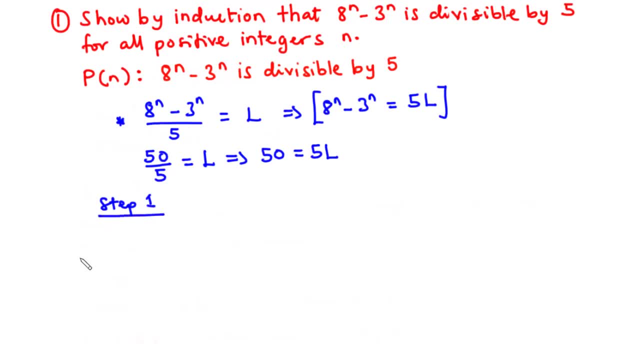 so for step 1, that is, the b step, we need to prove that the statement is true for the first term, that is, when n is equal to 1.. so for n equals 1, we have p of 1. so at this point we are going to substitute 1 in place of n in the original statement. so that is. 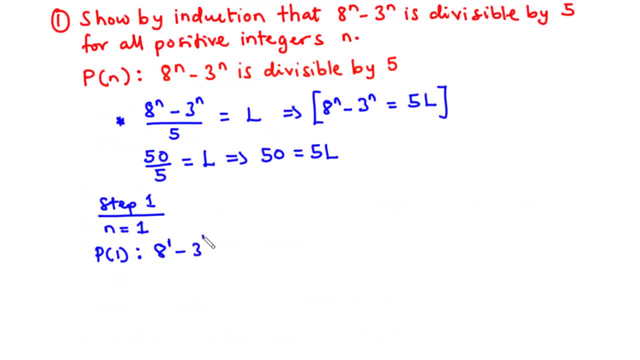 8 exponent 1 minus 3 exponent 1, and that is equal to 8 minus 3, and that is equal to 5.. now, since 5 is divisible by 5, we say that p of 1 is true. because we have 5 and that is divisible by 5, we have an integer value, say one, therefore p. 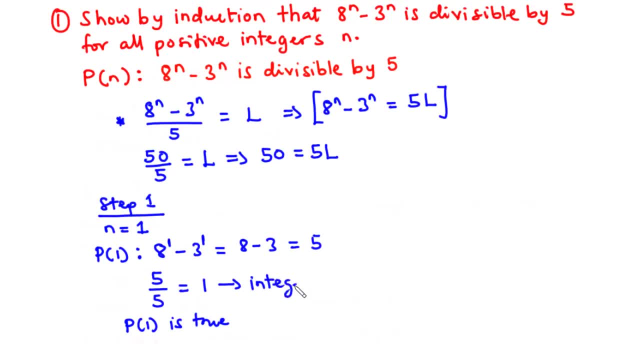 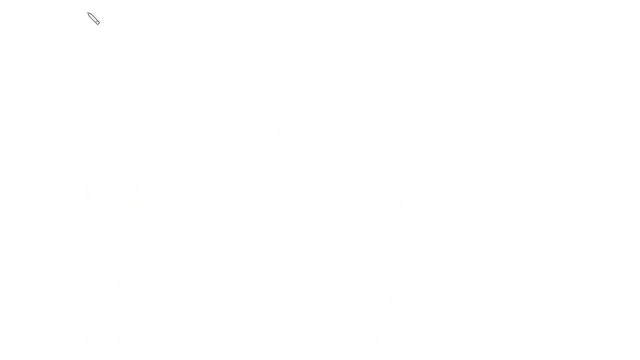 of 1 is true. now let's move on to step 2. that is where we are going to assume that the statement is true, for n equals k where k is any any positive integer. So for step 2, we have p, and then we are going to substitute. 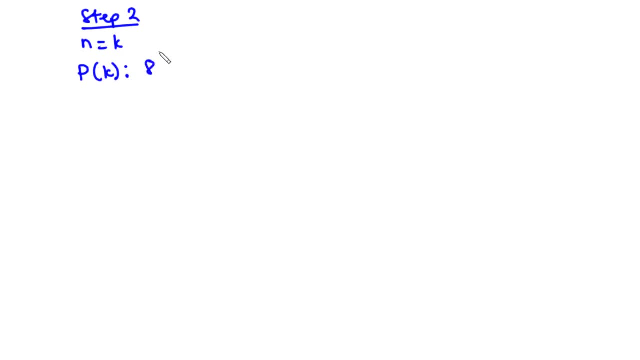 k in place of n. So we have 8 exponent k minus 3 exponent k, and we are assuming that this is equal to 5 times some integer value, say m. Now at this point let's make 8 exponent k the subject. So we have 8 exponent k equals 5m, and then we transpose this to the right. 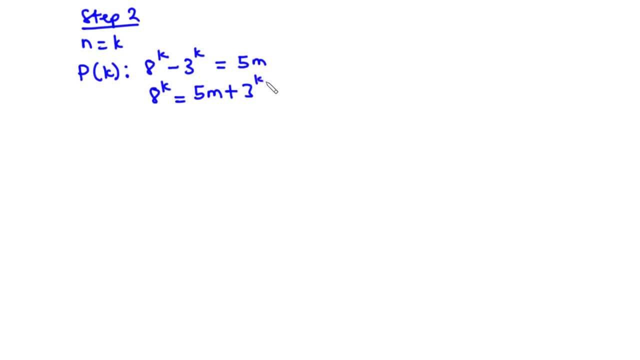 hand side, we have plus 3 exponent k. Now let's call this equation 1.. Now to step 3.. Here is where we are going to prove that the statement is true for the next time. that is n equals k plus 1.. So we have n equals k plus 1.. So p of k plus 1.. So that's going to be. 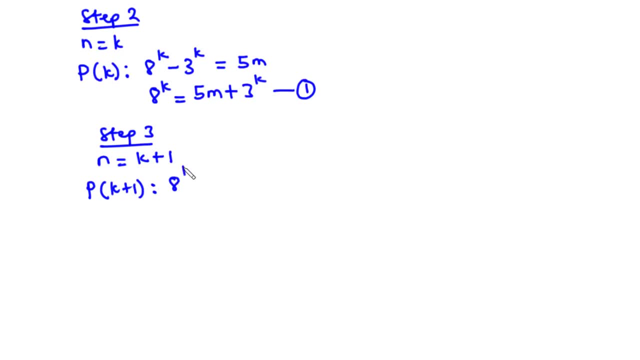 8 exponent. So we have 8 exponent. k plus 1 minus 3 exponent. k plus 1 equals 5 times some integer integer value, say L. At this point let's resolve the terms on the left hand side. So on the left hand side we have 8 exponent. 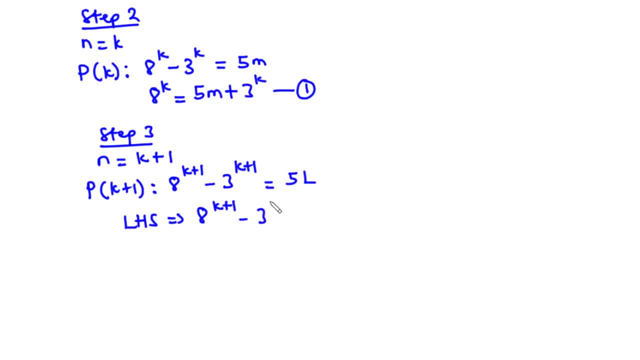 k plus 1 minus 3 exponent k plus 1.. So according to the laws of indices, we can resolve this as: 8 exponent k times 8 exponent 1 minus 3 exponent k times 3 exponent 1.. Now this is equal to 8 times 8 exponent k minus 3 times 3 exponent k. 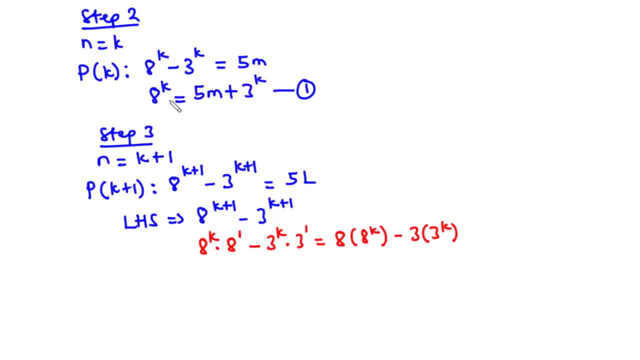 Now from equation 1, we have 8 exponent k equals 5m plus 3 exponent key. So we are going to substitute this in here. So that's going to be 8 times 5m plus 3 exponent key, minus 3 times 3 exponent key. Now let's multiply 8 across. 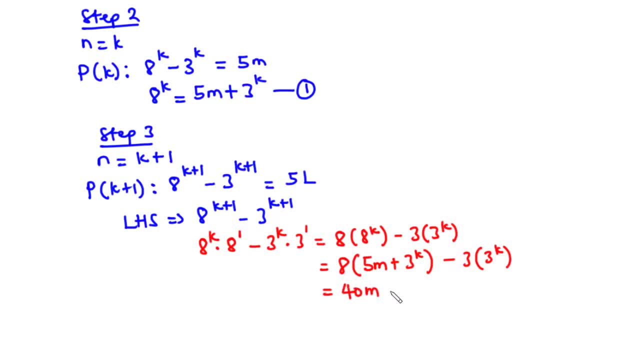 So that becomes 40m plus 8 times 3 exponent key, minus 3 times 3 exponent key. So at this point we have like things So we can simplify that. So that is equal to 40m. 8 minus 3 is 5.. So plus 5 times 3 exponent key. 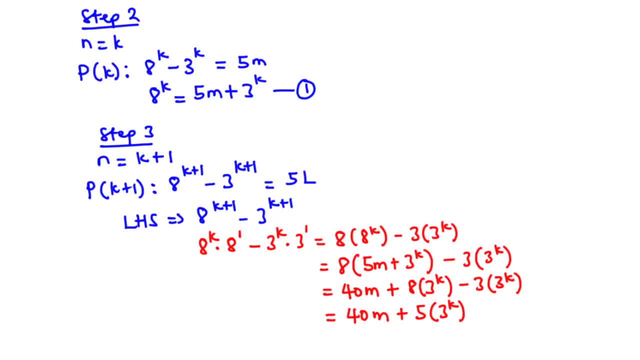 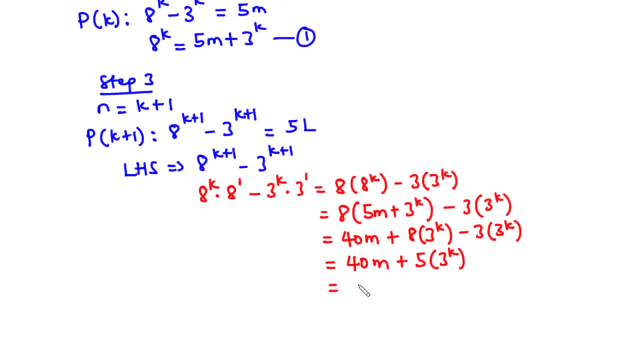 Now, since we are to prove that the original statement is divisible by 5, we are going to factor out 5.. So we factor out 5 so that we have: 40m divided by 5 is 8m plus 5 times 3. 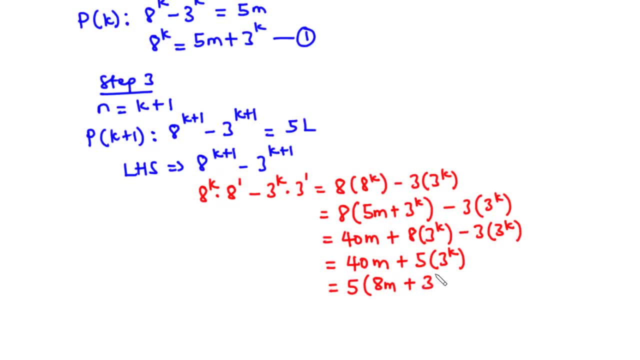 exponent key divided by 5 is 3 exponent key. So we have 5 into brackets, 8m plus 3 exponent key. Now we are going to let l equals 8m plus 3 exponent key And since m and k are both integers, it follows that l is also an integer In that case. 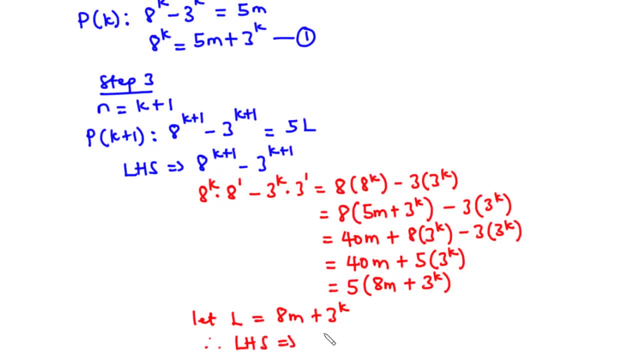 we have the left hand side to be 5 times l, and that is equal to the right hand side. So since the left hand side is equal to the right hand side, then we can say that the expression 8 exponent k plus 1 minus 3 exponent k plus 1 is divisible by 5.. Hence the original equation. 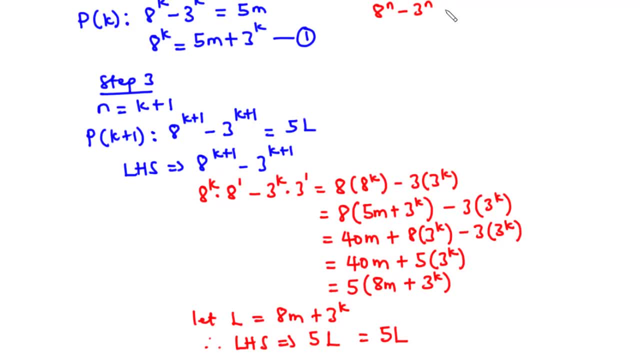 8. exponent n minus 3. exponent n is divisible by 5 for all positive integers n. Thus p of n is divisible, and 5 for the positive integers p of n n is true. for all positive integers n is greater or equal to 1.. 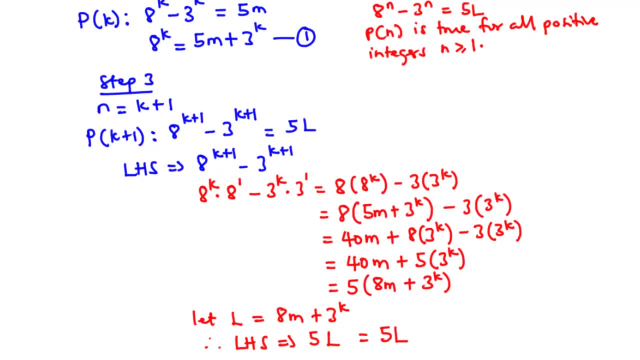 Now we can test our solution by substituting any value of n into the original equation. So let's assume that we have n equals 4.. Now if n is equal to 4, then from the original equation we have 8 exponent, 4 minus 3 exponent. 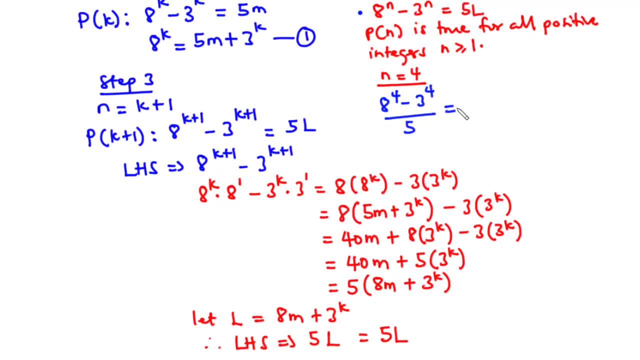 4 divided by 5, and this should be equal to some integer value. say l Now 8. exponent 4 is 4096 minus 3, exponent 4 is 81. So we divide by 5 and then we have l equals 4.. 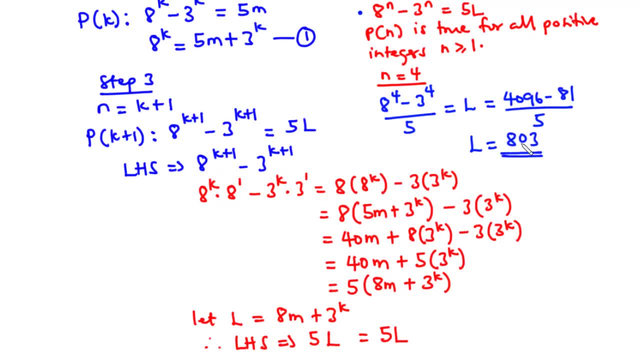 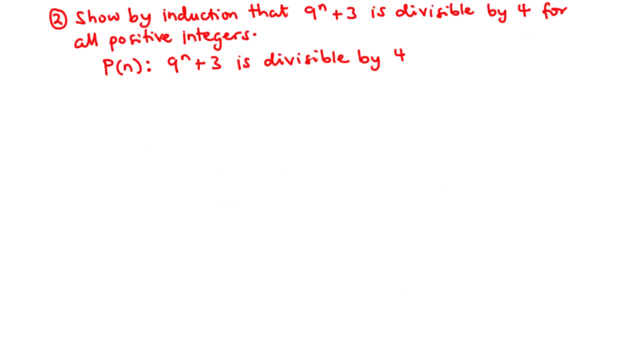 Therefore p of n is true for all positive integers. n is greater or equal to 1.. Now let's try the next problem. So for problem 2, show by induction that 9 exponent n plus 3 is divisible by 4 for all. 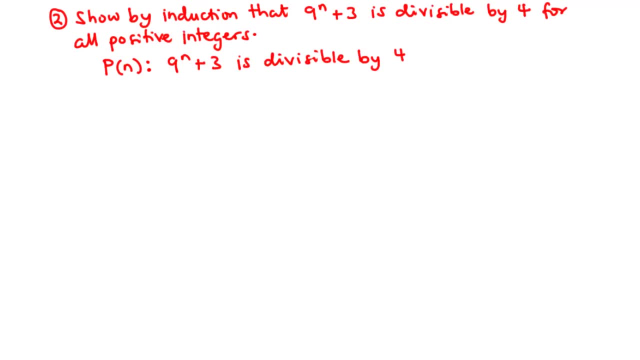 positive integers. So, given the statement, 9 exponent n plus 3 is divisible by 4.. First of all we need to prove that the statement is true for the first term, that is, when n is equal to 1.. So for step 1, we have: when n equals 1, we have p of 1, that is 9 exponent 1 plus 3, and 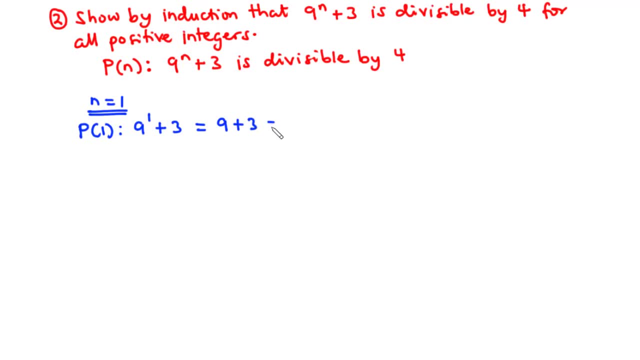 that is equal to: 9 plus 3 equals 12.. Now, since 12 is divisible by 4.. We say that 9 plus 3 equals 12.. Now, since 12 is divisible by 4.. We say that p of 1 is true. 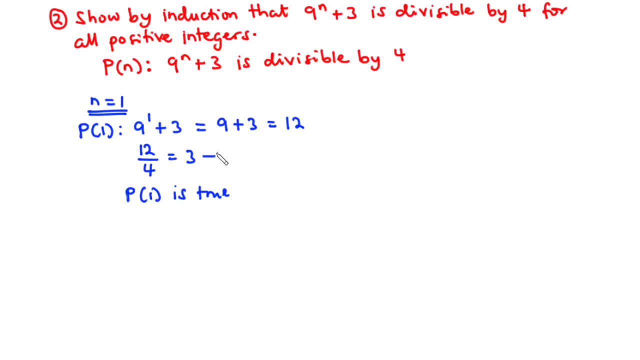 So 12 divided by 4 is equal to 3, where we have 3 to be an integer. Now to the second step. we are going to assume that the statement is true for n equals k where k is any positive integer. So we have p of k. 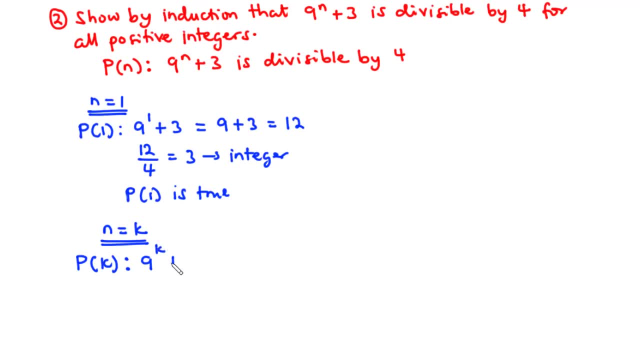 And that is 9 exponent n plus 3.. And that is 9 exponent k plus 3, equals 4 times some integer value, say m. Now, at this point we are going to make 9 exponent k the subject. So we have 9 exponent k equals 4m. 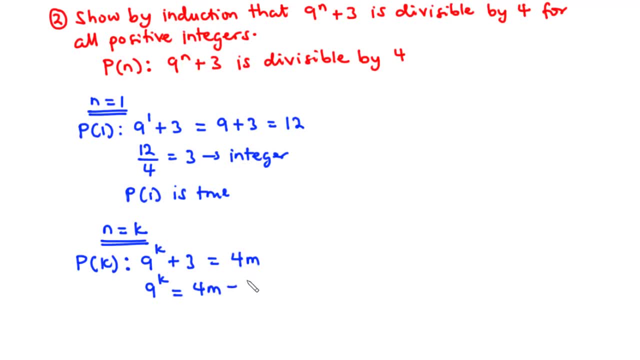 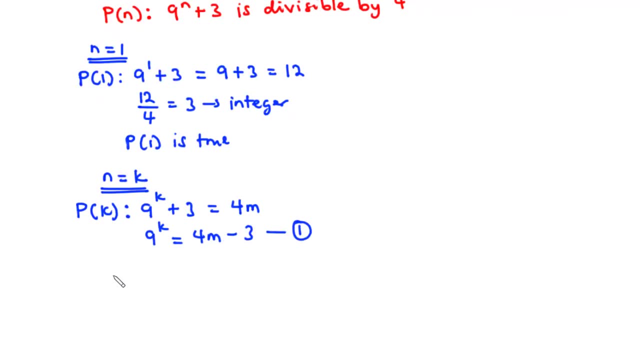 We transpose 3 to the right hand side, That becomes negative 3. We call this equation 1.. Now to the last step. We have 9 exponent k plus 3 equals 4 times some integer. Now, at this point we are going to prove that the statement is true for the next step. 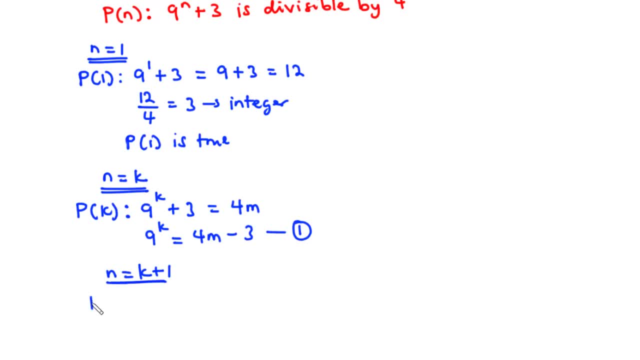 That is when n is equal to k plus 1.. So we have p of k plus 1.. Now, in place of n, we are going to substitute k plus 1. So we have 9 exponent. k plus 1 plus 3 equals 4 times 7.. 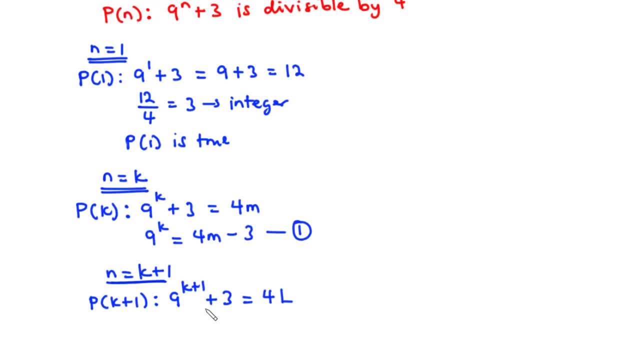 some integer value, say L. Now let's expand this. So that's going to be 9 exponent K times 9. exponent 1 plus 3 equals 4L. Now let's resolve the left hand side. So for the left hand side we have 9 times 9 exponent K plus 3, and that is equal. 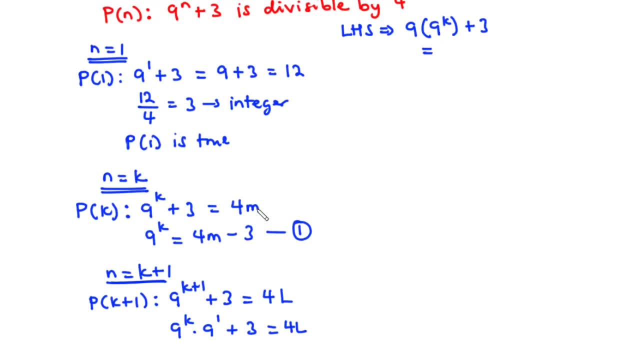 to 9. exponent K from equation 1 is 4M minus 3.. So we have 9 times 4M minus 3 plus 3.. Let's multiply 9 exponent K 9 across, So that becomes 36m minus 27 plus 3.. And we can simplify this as 36m minus 24.. 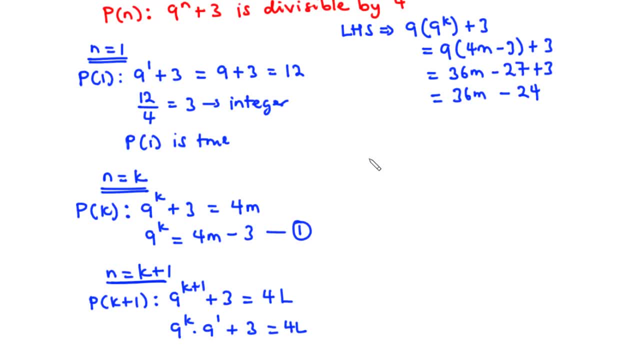 Now, since the original statement is divisible by 4, we are going to factor out 4.. So we have this simplified as we factor out 4.. 36m divided by 4, we have 9m minus 24. divided by 4 is 6.. At this point, we are going to let L equals 9m minus 6.. Simply because, since 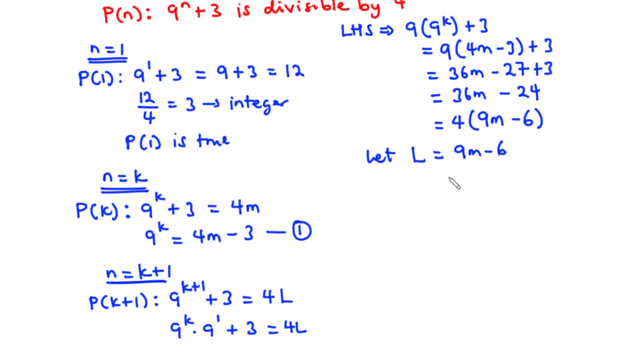 m is an integer, it follows that L is also an integer. Therefore, we have the left hand side to be 4 times L. Now, since the left hand side is equal to the right hand side, that is 4L equals 4L. we say that the expression 9, exponent k plus 1 plus 3 is divisible. 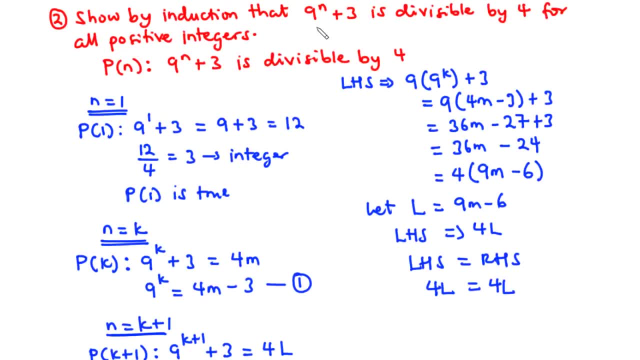 by 4.. Hence the original statement: 9 exponent k plus 1 plus 3 is divisible by 4.. Hence the original statement: 9 exponent k plus 1 plus 3 is divisible by 4.. Hence the original statement: 9 exponent k plus 1 plus 3 is divisible.